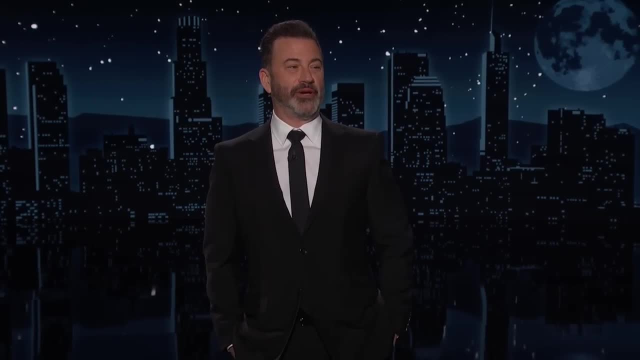 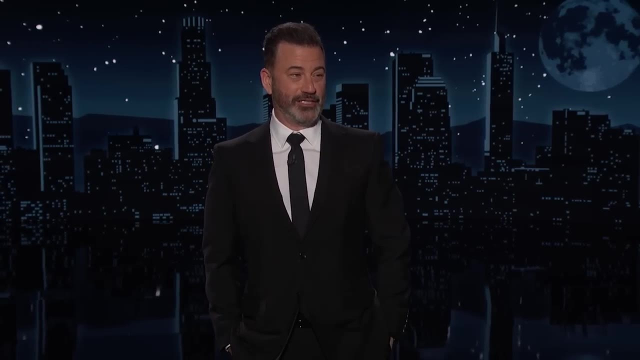 Trump is suing the judge in the trial for issuing a gag order that would prevent him from, among other things, attacking the judge's daughter, which he has done. This gag order is for the Stormy Daniels hush money case. It sounds like something out of an episode of Seinfeld. 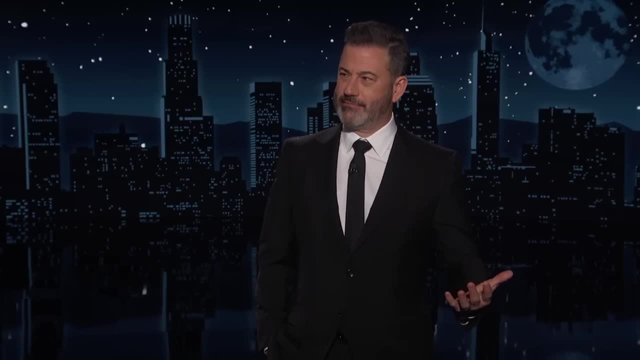 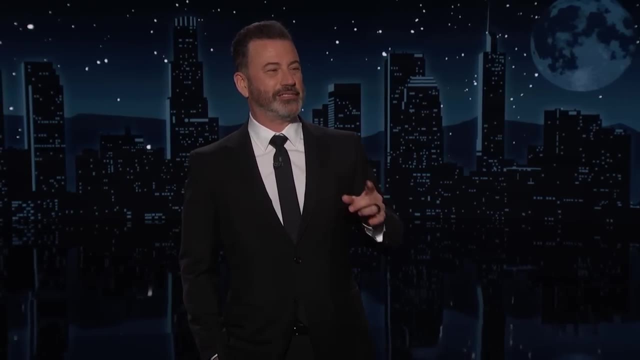 There's a gag order in the hush money trial. Can you gag a hush? Oh, you can gag a hush for sure. You know how many lawsuits Trump has been involved in. According to USA Today, four thousand ninety five. 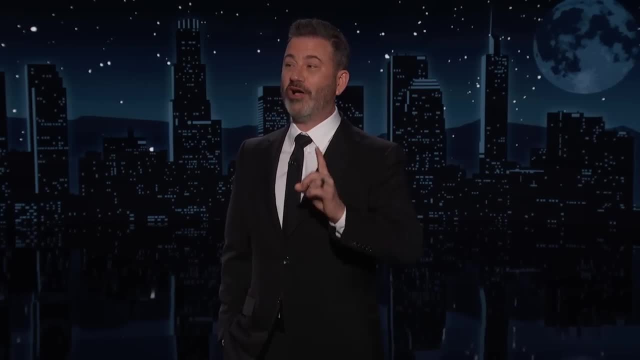 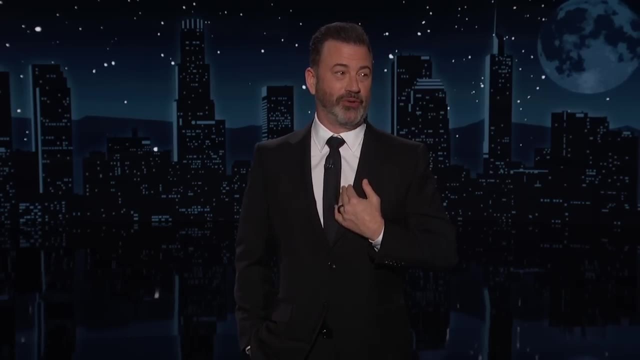 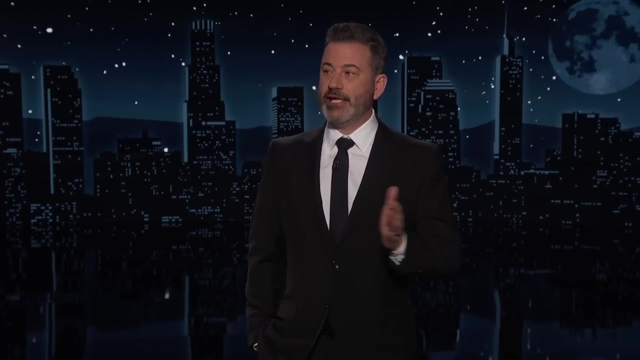 Before he was president. that's one lawsuit a day for eleven years. I say: if you get sued more than a hundred times in your life, we send you to Guantanamo Bay and that's it. But there has to be a maximum. He's doing everything he can to delay this hush money trial, which is what innocent people do, right. 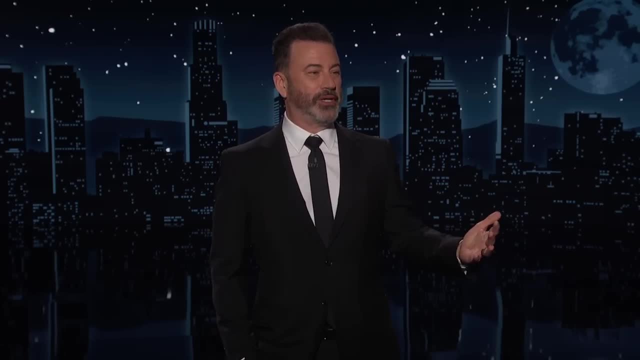 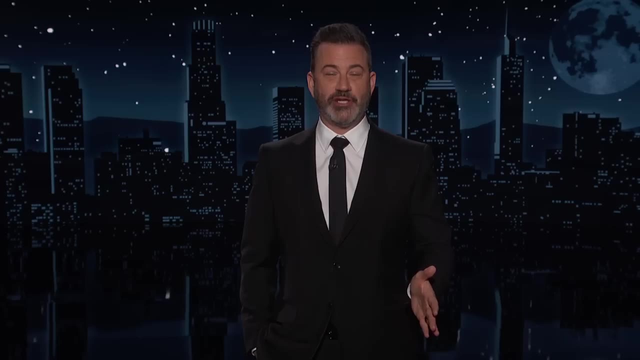 It's pure desperation. His team's down 15 points with two seconds left and they're still fouling in the game. The jury selection is expected to start on Monday. The judge yesterday released the questionnaire that they're going to use to vet potential jurors. 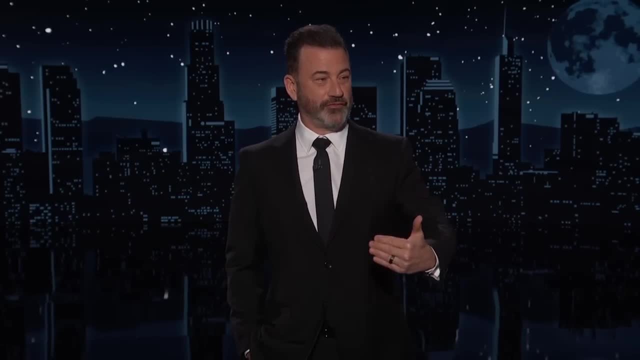 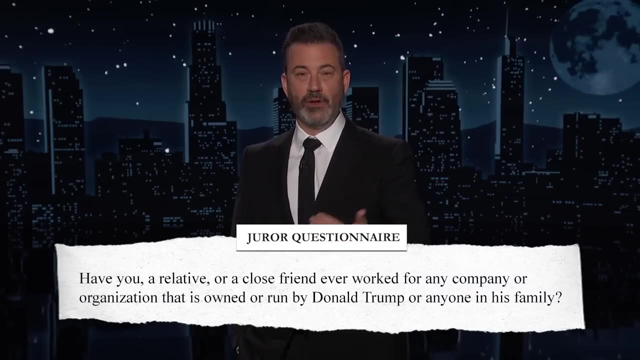 You know they're not allowed to directly ask the jurors who they voted for, but they can get information in roundabout ways, And these are some of the ways they ask: Have you a relative or a close friend ever worked for any company or organization that is owned or run by Donald Trump or anyone in his family? 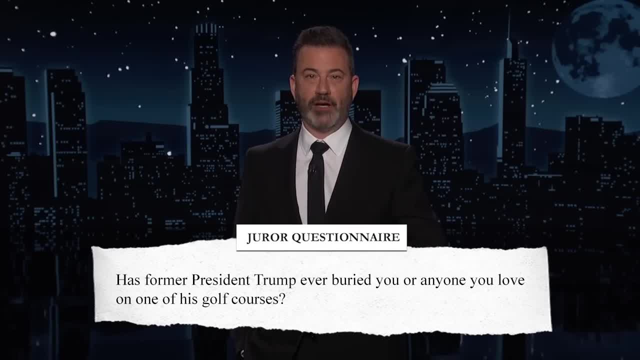 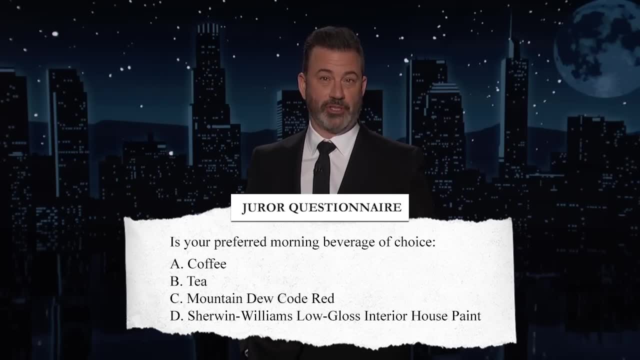 Has former Trump ever buried you or anyone you love on one of his golf courses? Is your preferred morning beverage coffee, tea, Mountain Dew Code Red or Sherwin-Williams low-gloss interior house paint? Have you ever had sex with Donald Trump? 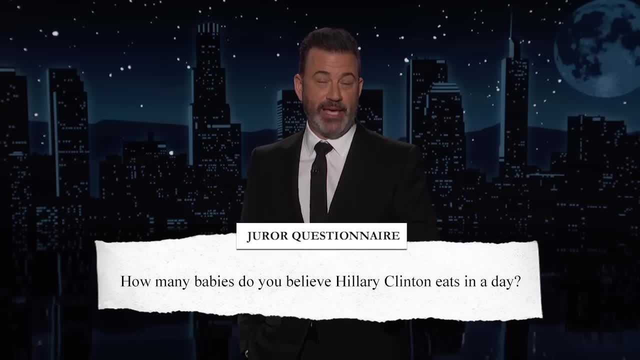 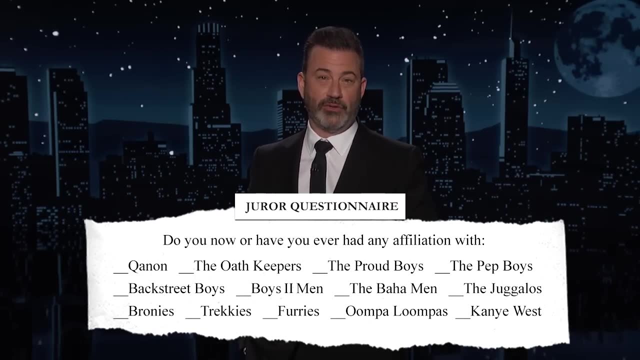 If yes, for how many seconds? How many babies do you believe Hillary Clinton eats in a day? And do you now, or have you ever, had any affiliation with QAnon, the Oath Keepers, the Proud Boys, the Pep Boys, Backstreet Boys? 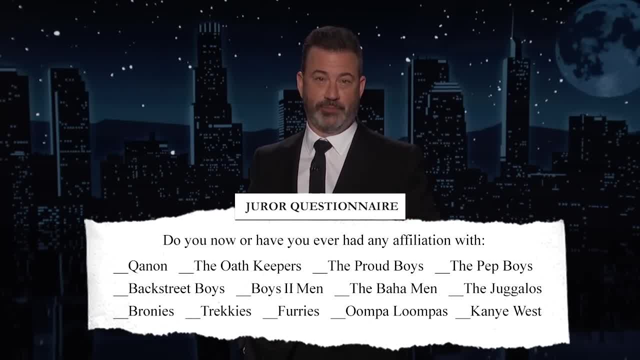 Boyz II Men, the Baja Men, the Juggalos, Bronies, Trekkies, Furries, Oompa Loompas or Kanye West. If you have an answer to those, you may or may not. 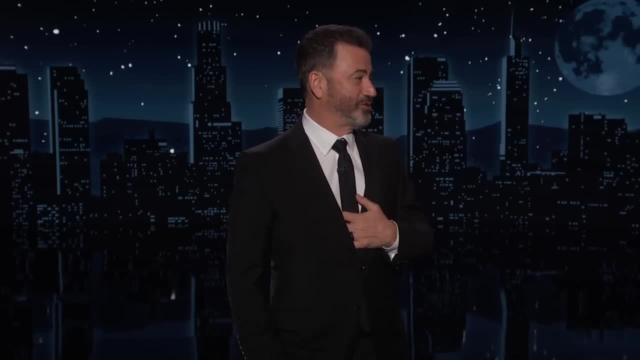 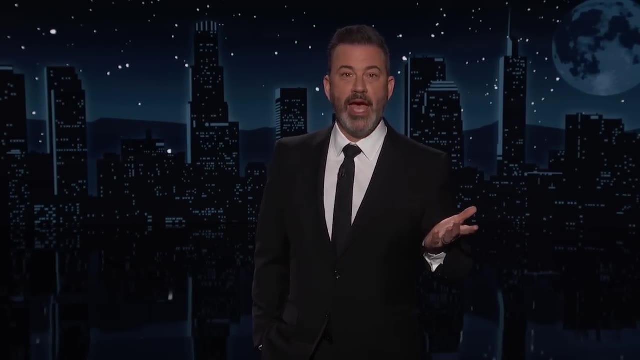 I wish I could get in on questioning these potential jurors. I feel like I'd be so good at it. And one final question, sir: Does your truck have nuts? And then we have the January 6th case in Washington, which hinges on a big hearing before the Supreme Court later this month. 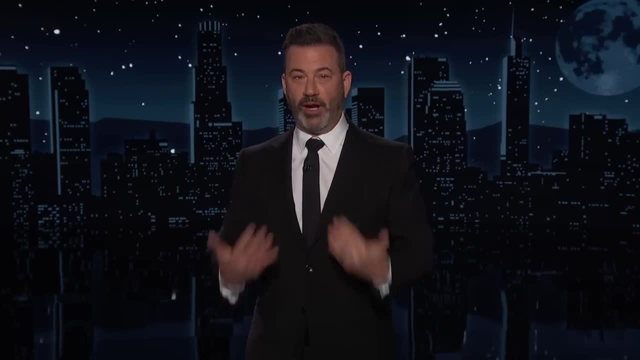 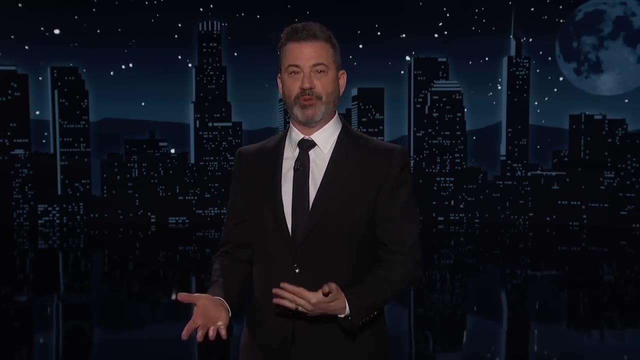 They will rule on Trump's silly claim that he can't be prosecuted because he had presidential immunity. The special counsel, Jack Smith, yesterday delivered his brief to the Supreme Court And just to make sure they read it, he delivered it in a brand new RV and left the keys behind. 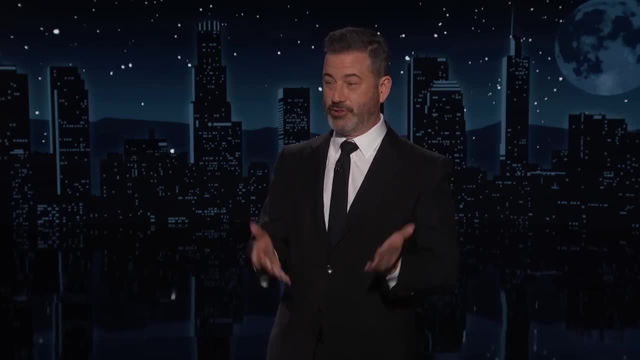 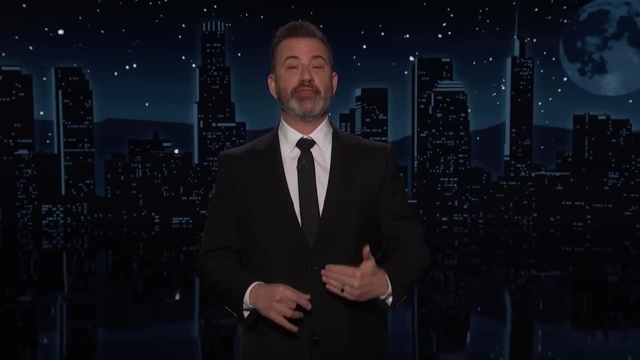 But Trump appointed three of those judges to the Supreme Court, which led to overturning Roe v Wade. But now he's saying he's not for a federal law against abortion. He thinks the decision should be left to the states. Trump believes that every woman should have the right to drive 600 miles for health care. 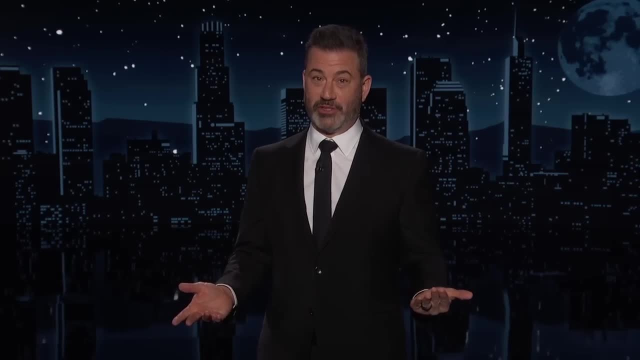 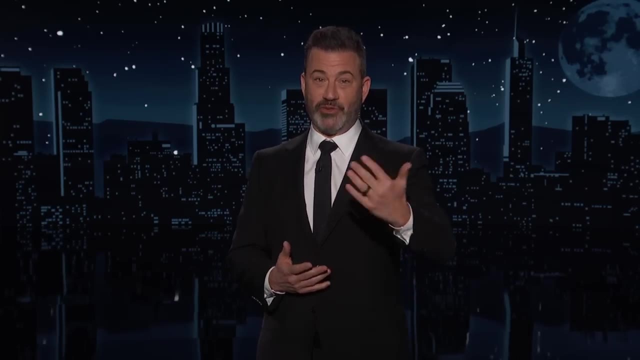 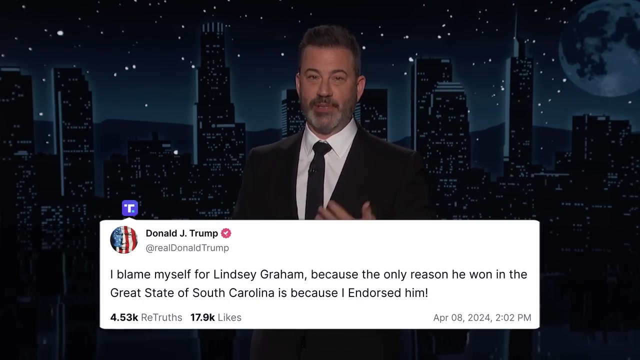 And this is now upsetting a lot of his supporters, including Senator Lindsey Graham, who said Trump's making a mistake- And that is not the kind of thing Trump likes to hear from his pals. So he lashed out. He wrote: I blame myself for Lindsey Graham because the only reason he won in the great state of South Carolina is because I endorsed him. 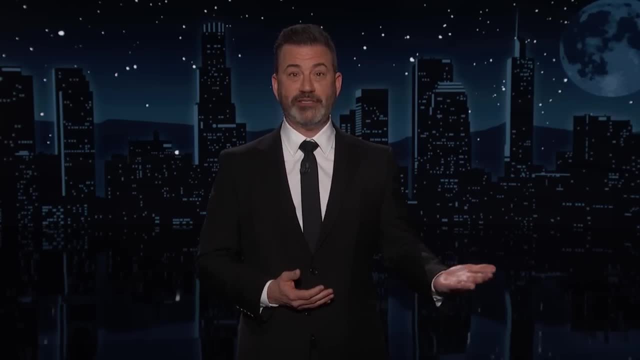 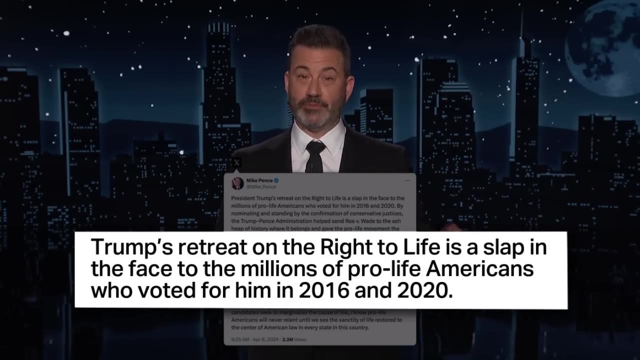 And then he got it from his former vice poodle too. Mike Pence wrote: Trump's retreat on the right to life is a slap in the face to the millions of pro-life Americans who voted for him. Trump did not respond to that. 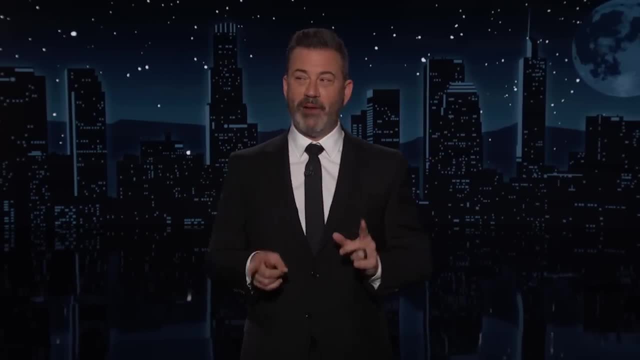 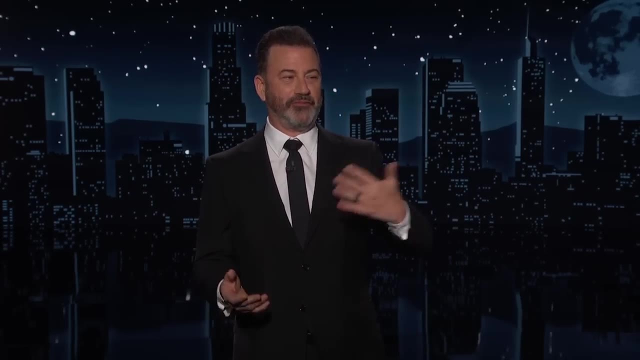 I think he's scared of Mike Pence He never responds to. I think Mike Pence must know too much is what's happening there. I think he's scared of Lindsey Graham. This is a game they're playing because seven out of ten of Americans believe women should have the right to choose. 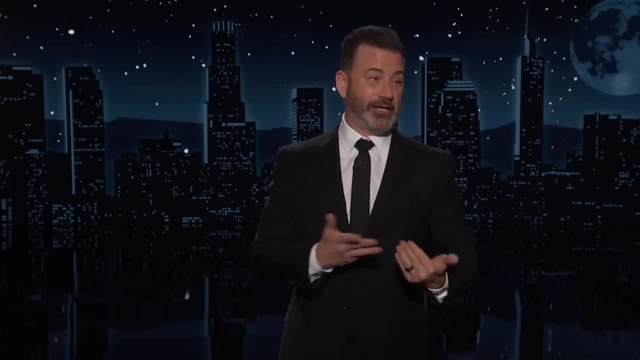 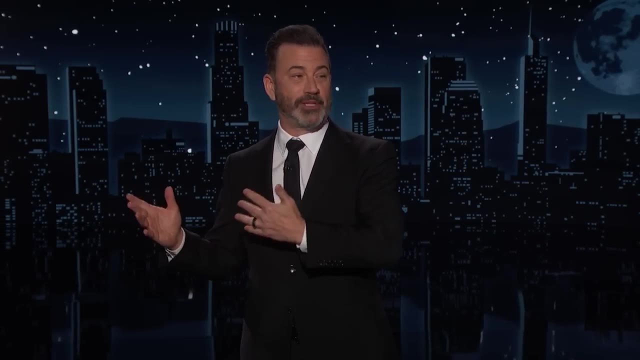 And Republicans are losing elections on this. So Trump is going to be the good guy or the bad guy, depending on which side you're on, And then Lindsey will be on the other side, fitting hissy saying Trump is too lenient to calm the pro-church Republicans down. 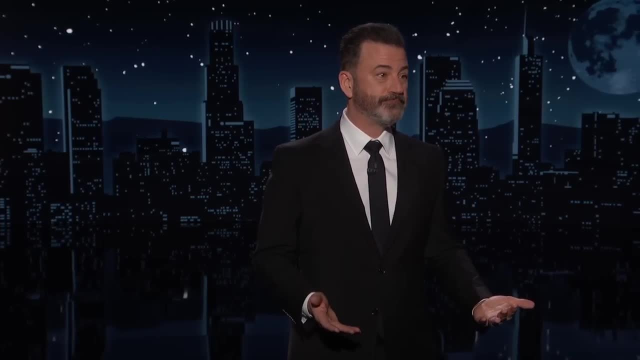 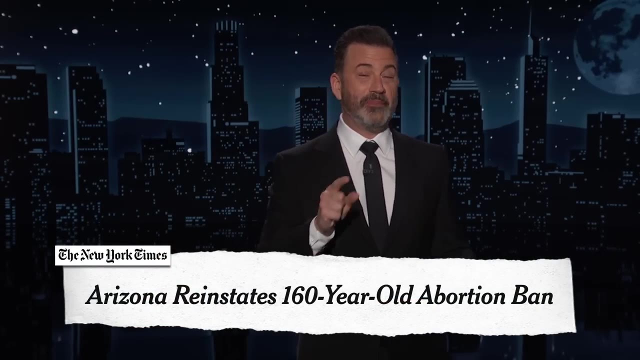 It's like wrestling, but with guys who, if you saw them in their underpants, you would throw up. Meanwhile, the Arizona Supreme Court today ruled that the state has to follow a law in 1864 that makes getting an abortion a criminal offense, with a sentence of two to five years in jail. 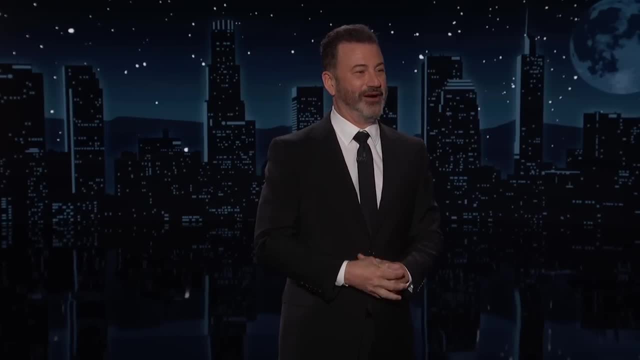 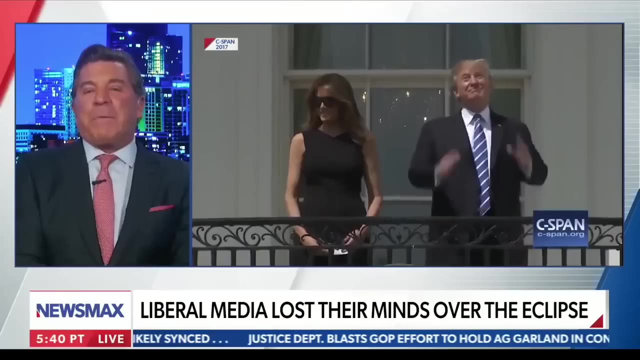 Isn't that great. We're playing by the 1864 rules now And these weaklings who worship Trump. everything he does is great. Even looking directly at an eclipse is great. Remember back in 2017, when people were criticizing President Trump for looking at the eclipse. 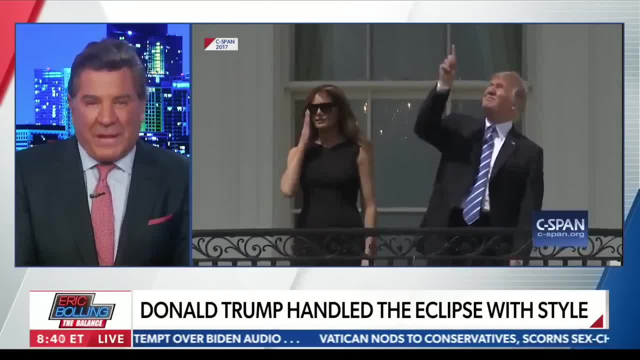 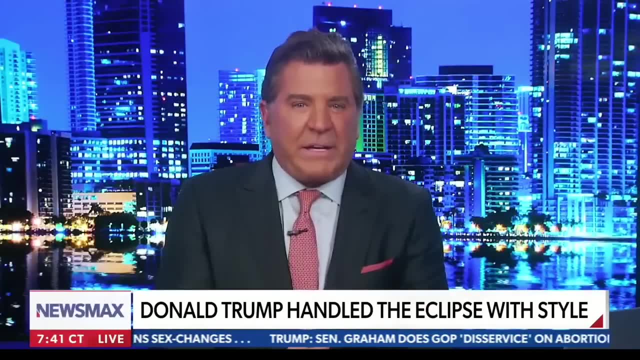 All of the things Donald Trump did that he was told not to do. looking up during the eclipse was the most on brand. That was hysterical, But I can relate. You can only say real men can look directly into an eclipse, right? 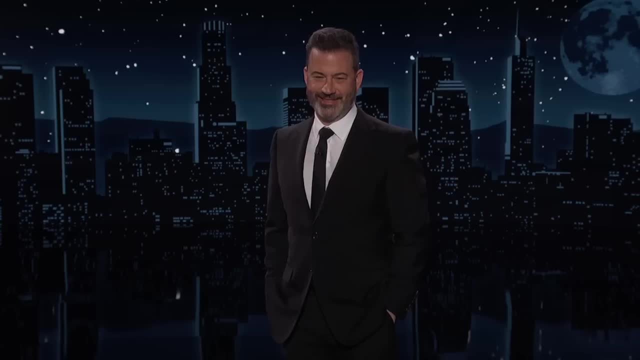 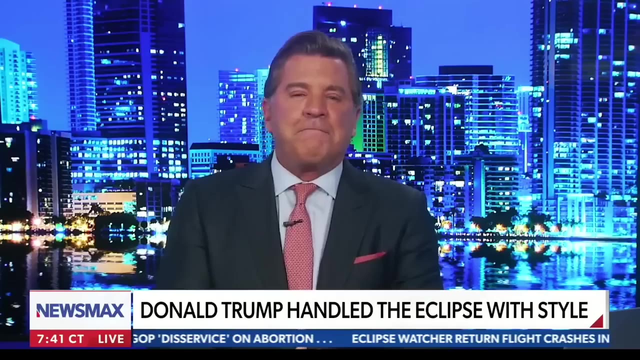 Just like when Hercules shot an arrow into the sun: Defiant- Yeah, defiant, By the way, look at this line at the bottom of the screen: Donald Trump handled the eclipse with style. And Grace, don't forget Grace, He handled the eclipse with style. 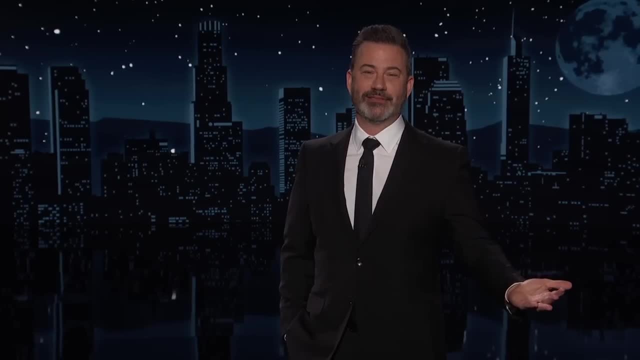 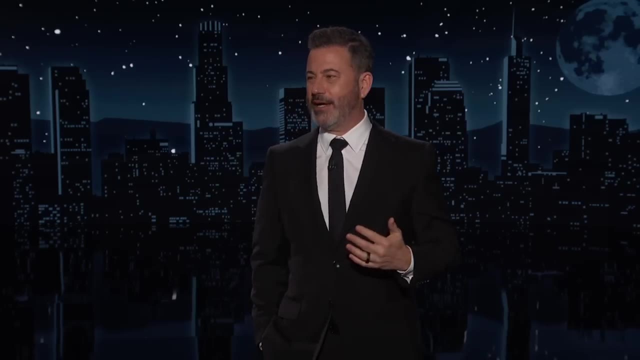 That big moron is lucky he isn't blind right now. How many of you went outside to see the eclipse yesterday? It was kind of I don't know, fun to have everybody looking up at the same time, But the other effect it had is it activated, the crazies. 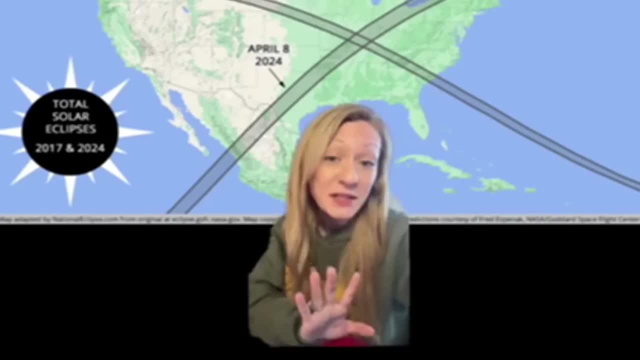 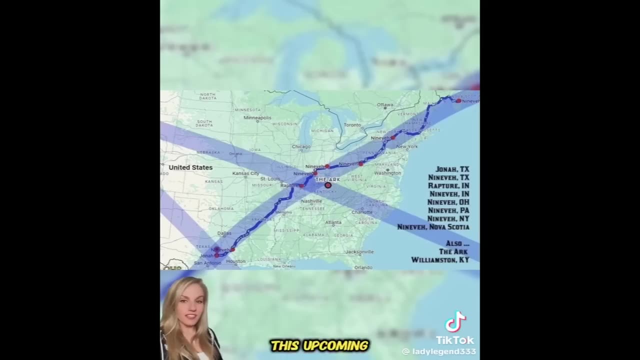 I'm telling you right now something is not right about this eclipse. This is the path that it will take, And it will cross over with the eclipse that we had in 2017, making an X on the country. This upcoming eclipse will also be going through Rapture Indiana. 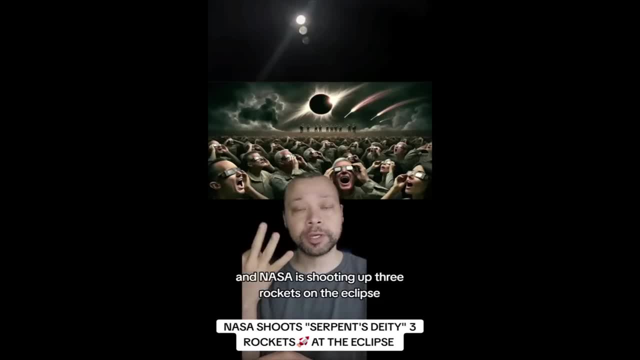 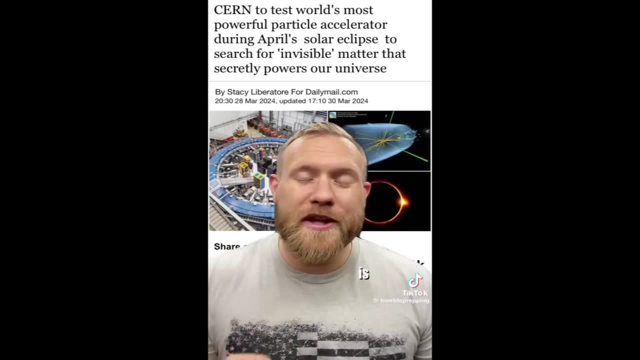 NASA is shooting up three rockets on the eclipse And guess what? they're calling it Serpent's Deity, And all the masses will be out with their glasses to watch it. What do you think is really going on with this Hadron Collider? 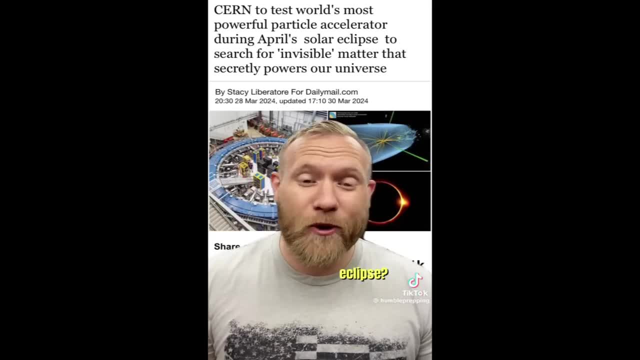 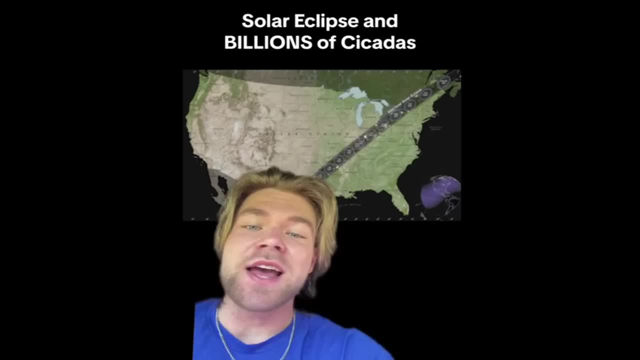 Hadron Collider tested at the same time as the solar eclipse, Something might come through the dimensional doors. A 10-year eclipse and a 10-year cicada hibernation has lined up perfectly on the hour. The fact that this hasn't ever happened before is suspicious. 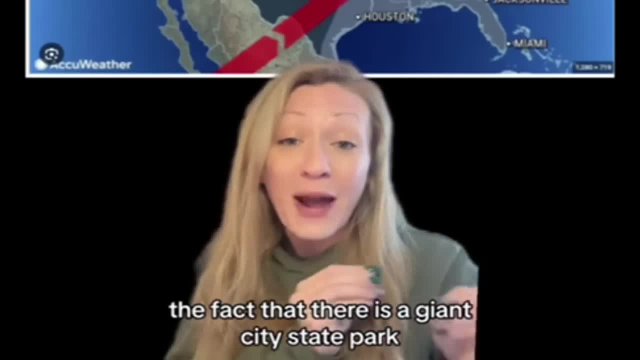 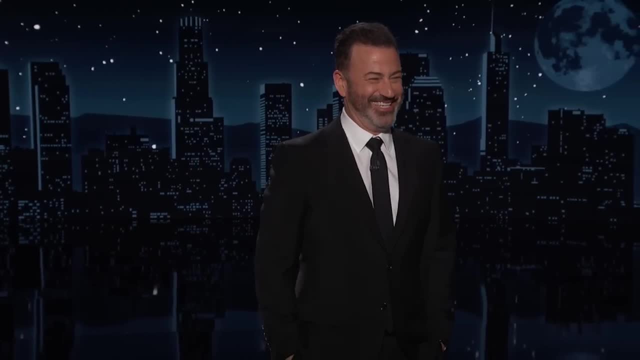 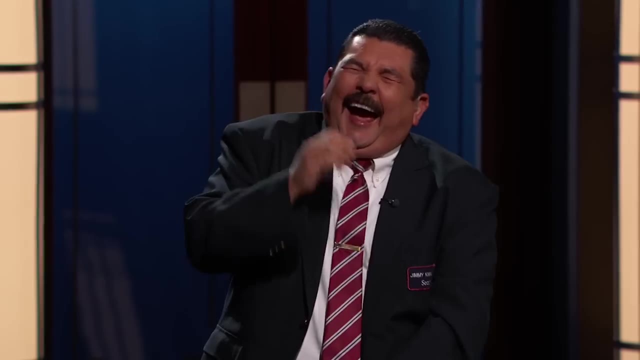 The fact that there is a giant city-state park right outside Sewanee National Forest, which is known for Bigfoot sightings, is suspicious. You ever seen a Bigfoot, Guillermo? No, You all right. Oh well, I don't want to. you know, I don't want to spoil your mood. but we got some sad news this weekend, especially for those of us here on the West Coast. I don't know if you heard: the 99-Cent Store filed for bankruptcy. They're closing all 371 stores for good. Apparently, the business model of we can never, ever raise the price of anything wasn't the best idea. 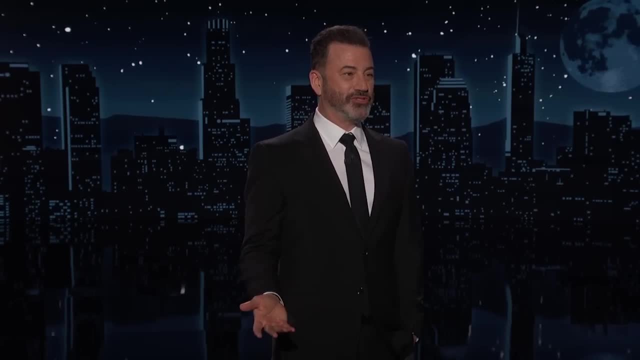 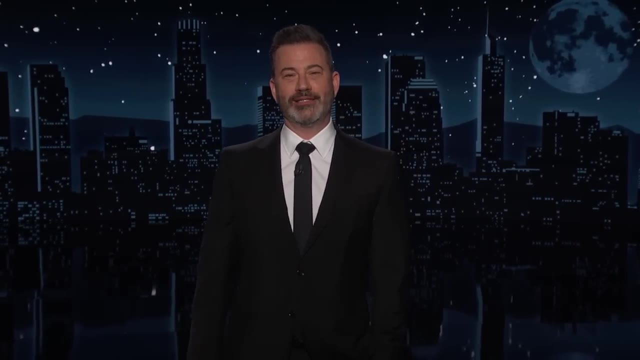 We have a lot of 99-Cent Stores. They're kind of an institution here And a lot of people in LA are bummed out. One of our writers, Jamie, texted her mom and she wrote: how do you feel about the 99-Cent Store closing? 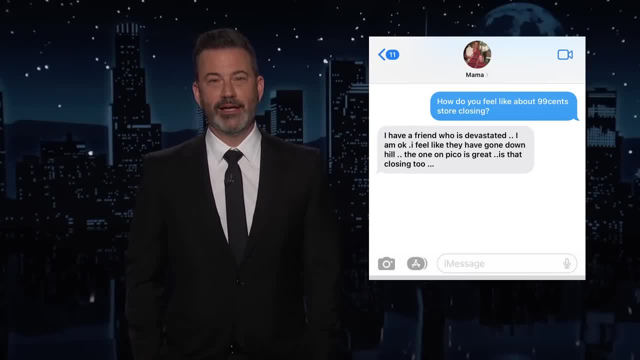 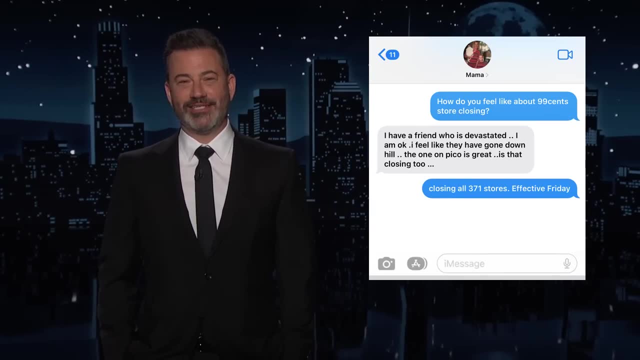 Her mom said: I have a friend who is devastated. I am okay. I feel like they've gone downhill. The one on Pico is great. Is that closing too? And Jamie said: closing all 371 stores effective Friday. Her mom said it is the end of an era. 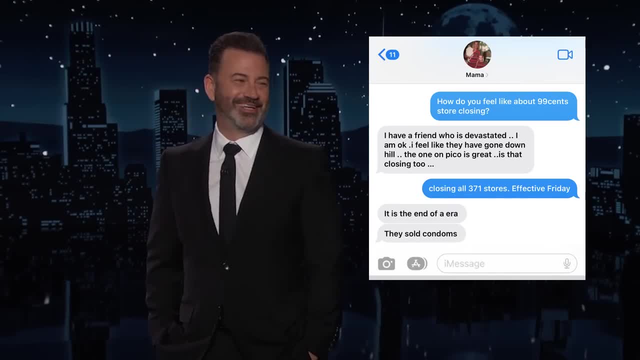 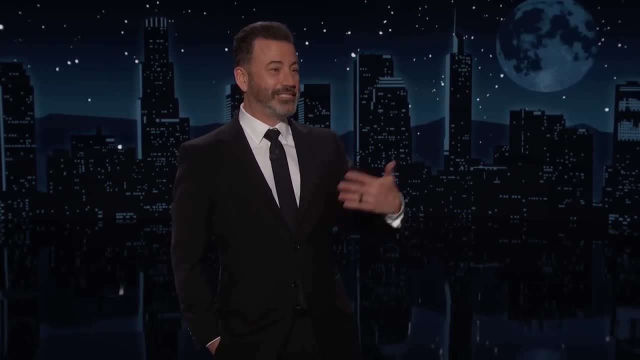 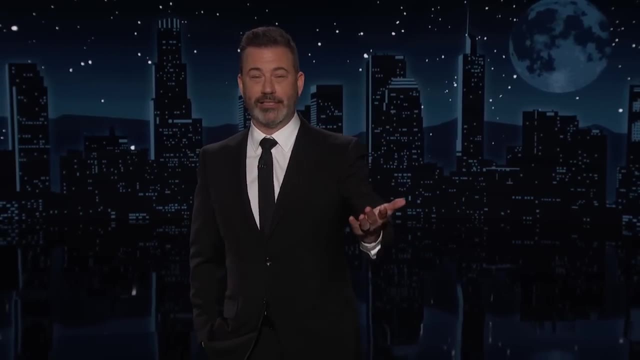 They sold condoms, which Not the best condoms, but they had them. So then we said: oh, this is funny. Let's ask other people who work here to text their mothers about the 99-Cent Store. And one of our editors, Kevin, said: how do you feel about the 99-Cent Store closing? His mom replied: I didn't hear. I use Dollar Tree anyway, but I think that sucks. I just got home from my procedure for my back. I'm very sore, Just have to rest, and the soreness can last up to three days before I start feeling relieved. 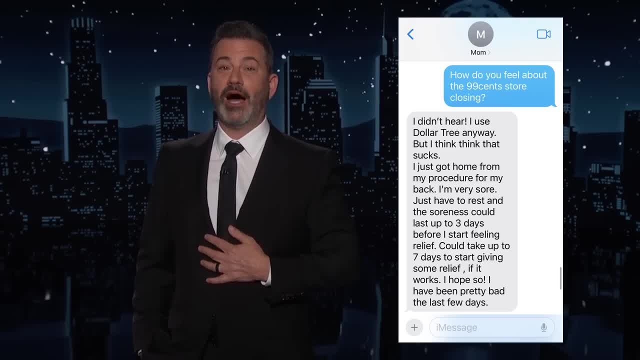 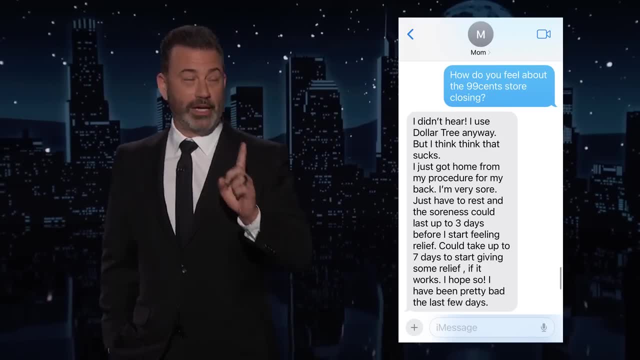 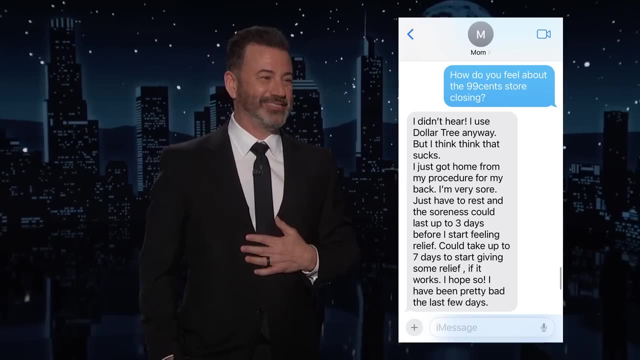 Could take up to seven days to start giving some relief, if it works. I hope so. I've been pretty bad the last few days. I think the message is two things. Number one: Kevin needs to be more in touch with mom And they probably sold some pretty good heating pads at the 99-Cent Store. 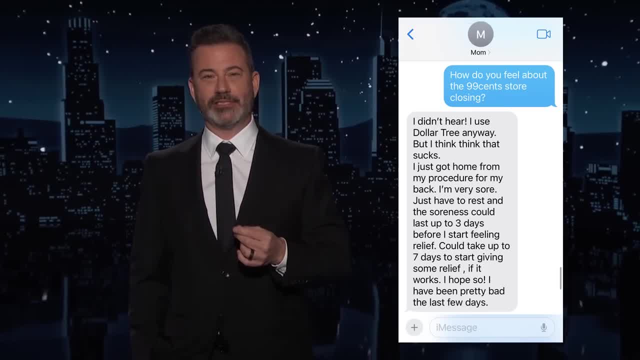 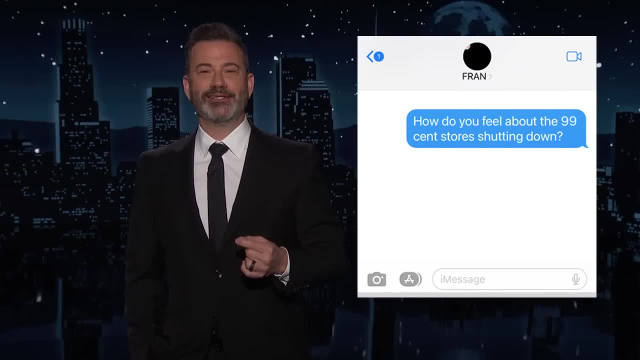 This is a response to Jillian, who's one of our executive assistants. Her mom said: she said: how do you feel about the circle? I need to stock up on sponges. My cousin Sal texted his mother. 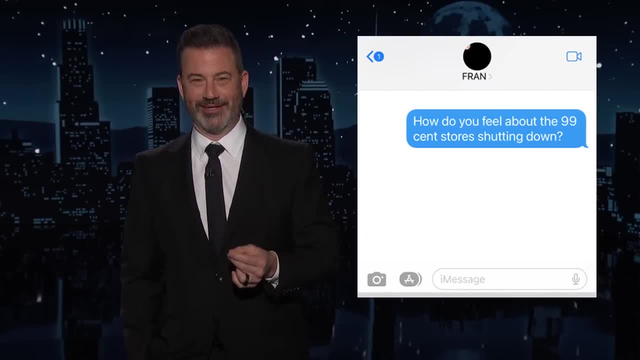 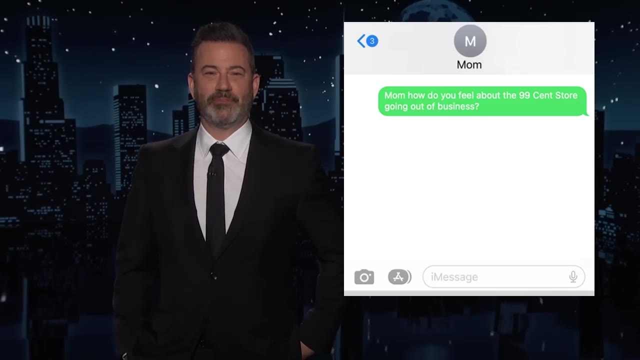 My Aunt, Fran. He said: how do you feel about the store shutting down? She said I'm brokenhearted. The only place I felt rich And I didn't have to hesitate, I just filled my cart. This is from one of our writers, Danny, who asked his mom how she feels about this. 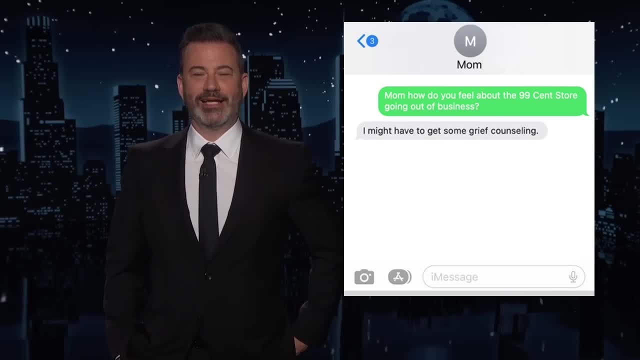 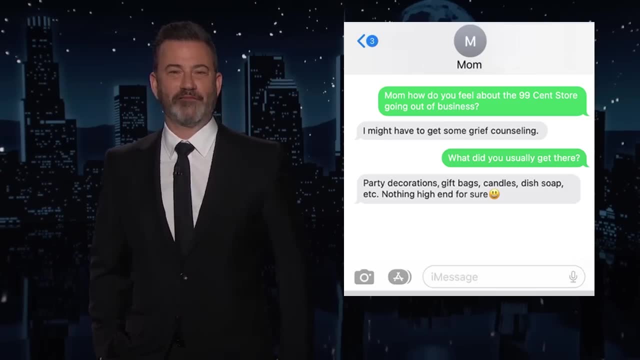 His mom said I might have to get some grief counseling. And then Danny was like: all right, what did you usually get there? She said: party decorations, gift bags, candles, dish soap, et cetera. Nothing high end, for sure. 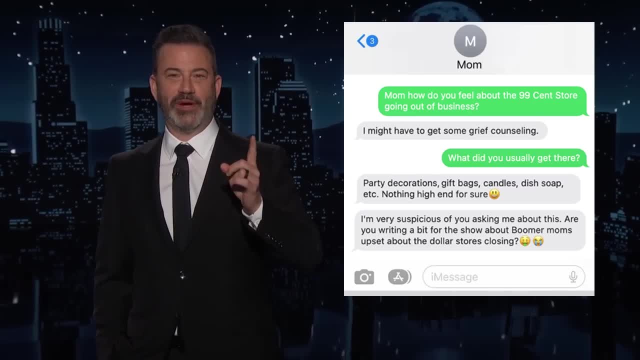 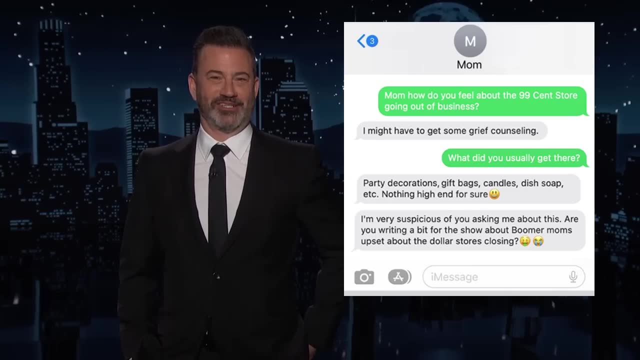 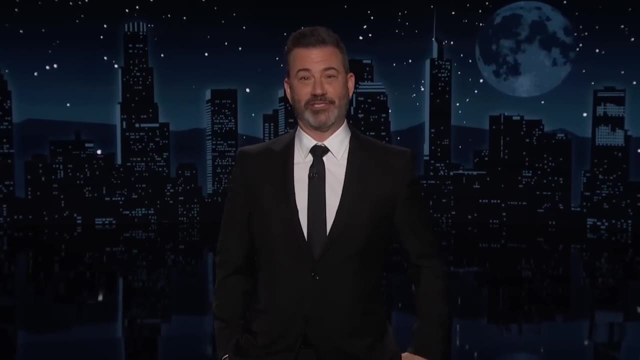 And then she wrote- I'm very suspicious if you ask me about this: Are you writing a bit for the show about boomer moms upset about the dollar store? It's the 99-Cent Store, not a dollar. And yes, we are, Mrs Ricker.